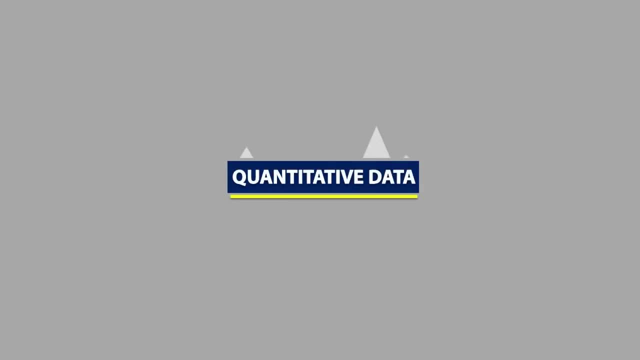 charts as a way of tallying information. For quantitative data, we often use stem plots, histograms and time plots to show information. We'll talk about histograms first. After collecting data from a population or sample, we can use a histogram to help us display. 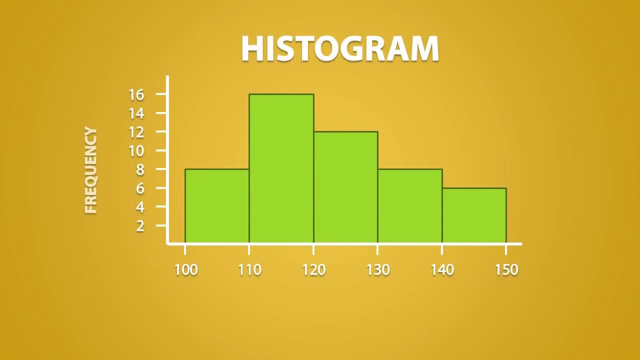 the distribution of the data we collected. The frequency, or count, is displayed on one axis, and each count tell us how many data values fall within a predetermined interval. on the other axis, This axis corresponds to the variable we have just measured. To read a histogram, you first pick one of the intervals and determine its height, For. 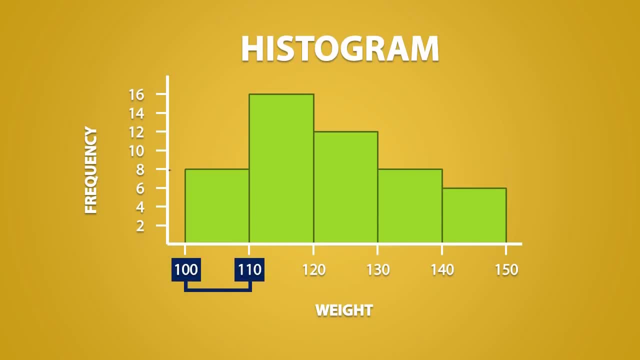 the interval between 100 and 110,, we see that the bar has the height of 8.. This means that, from the data we collected, 8 people weigh between 100 and 110 lbs pounds. For the next interval, we see that the bar has a height of 16, so this means that 16. 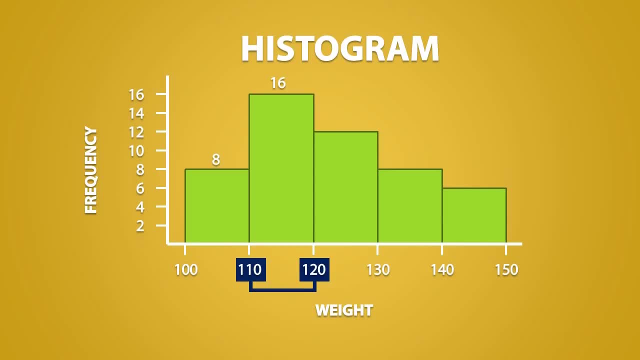 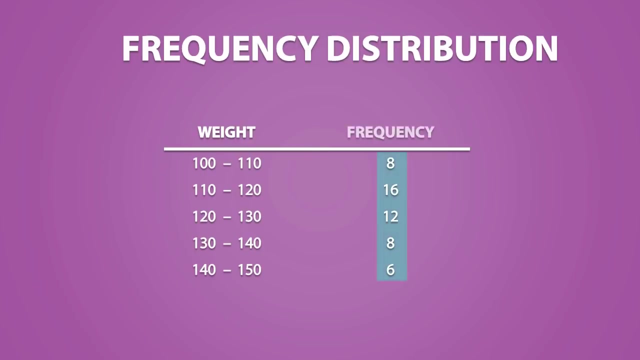 out of the total people I collected data from weigh between 110 and 120 pounds. The rest of the histogram can be read in a similar fashion. A histogram is a form of a frequency distribution. Frequency distributions can be written in a table format and they tell us how many. 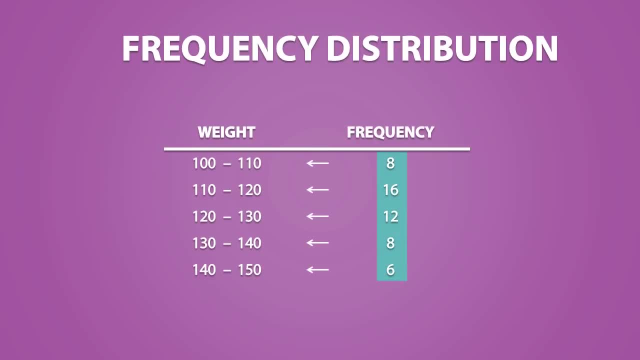 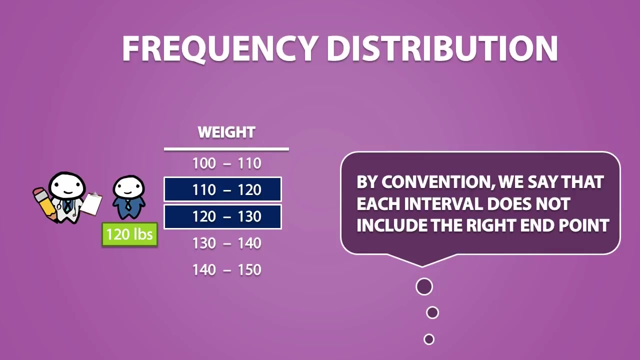 data values fall within a certain interval. These intervals can be a little confusing. For example, if I recorded an individual's weight to be exactly 120 pounds, do I include them in this interval or this interval? By convention, we say that each interval does not include the right endpoint. 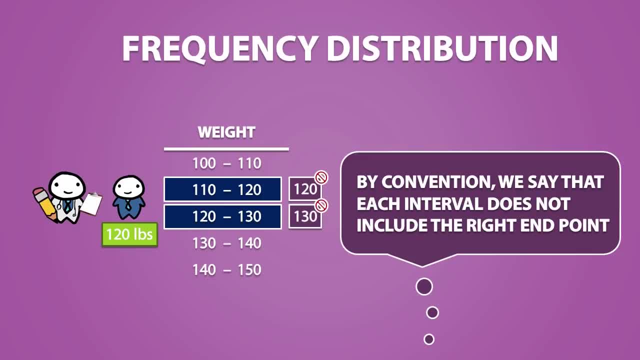 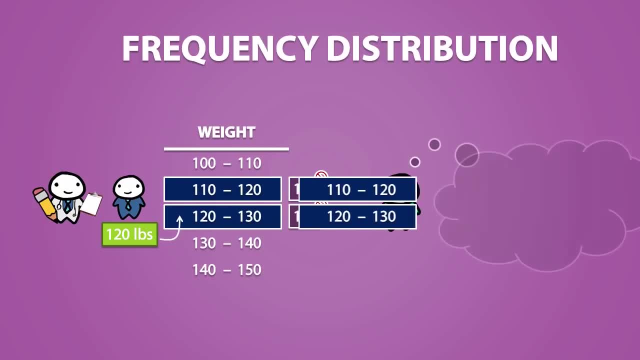 So 120 is not included in this interval and 130 is not included in the other interval. So in fact, 120 belongs to the second interval. Now you might be thinking: if the right interval isn't included, why do I have to include? 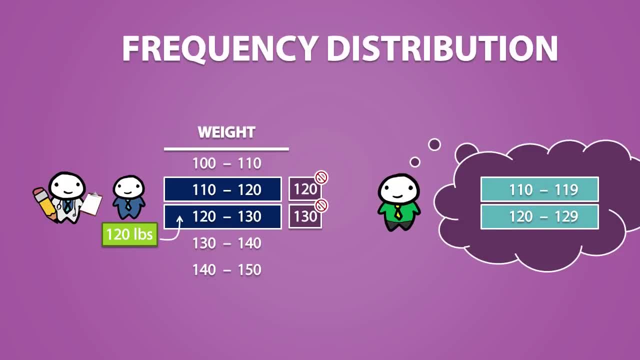 it? Why don't I just rewrite my intervals like this: 110 to 119, and 120 to 129?? Now, the problem with this is that we don't have continuity. For example, if you weighed 119.7 pounds, there would be no interval that contains this. 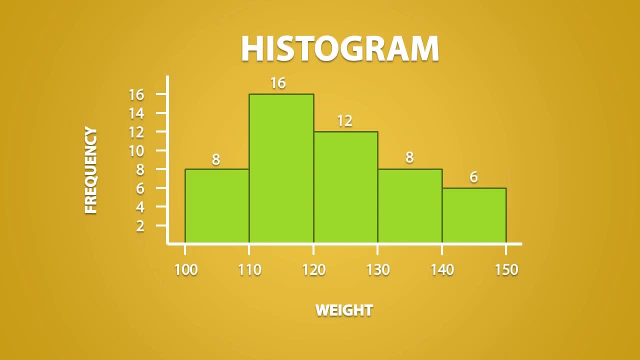 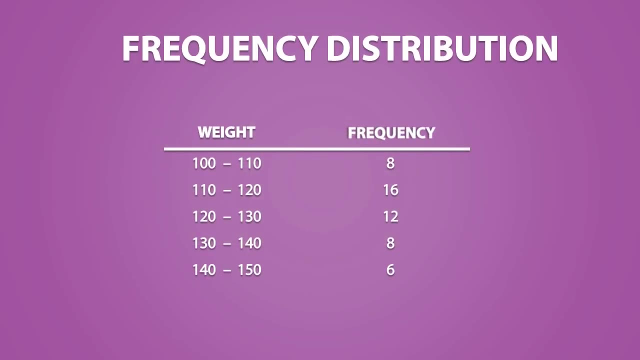 The rest of the histogram can be read in a similar fashion. A histogram is a form of a frequency distribution. Frequency distributions can be written in a table format, and they tell us how many data values fall within a certain interval. These intervals can be a little confusing. 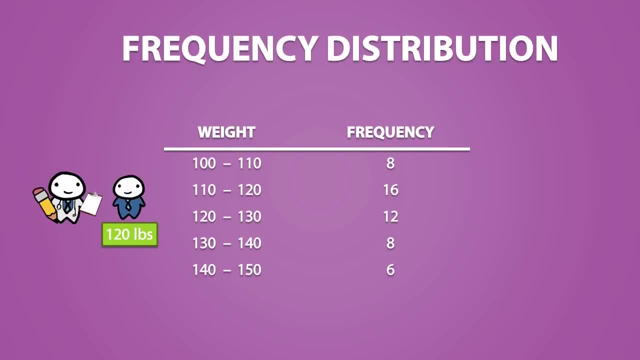 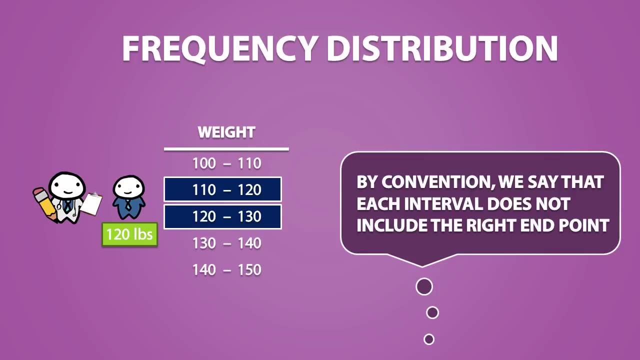 For example, if I recorded an individual's weight to be exactly 120 pounds, do I include them in this interval or this interval? By convention, we say that each interval does not include the right endpoint. So 120 is not included in this interval and 130 is not included in the other interval. 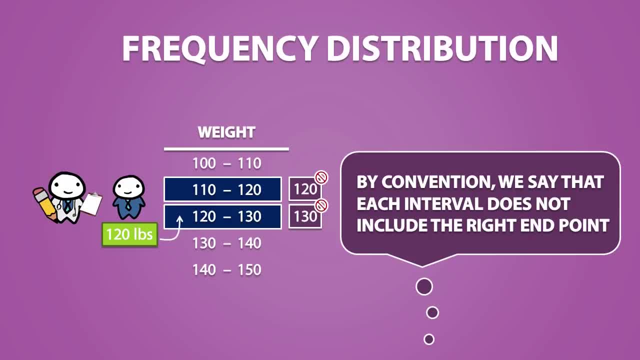 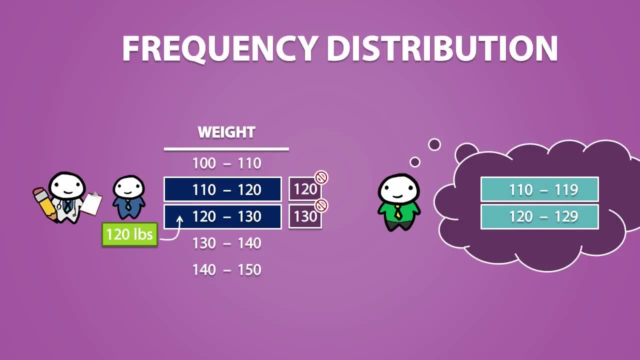 So in fact, 120 belongs to the second interval. Now you might be thinking: if the right interval isn't included, why do I have to include it? Why don't I just rewrite my intervals like this: 110 to 119, and 120 to 129?? 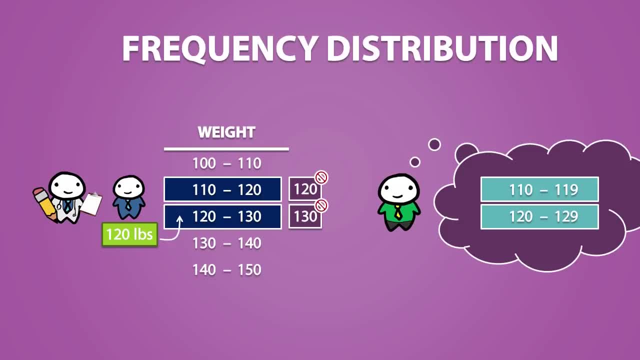 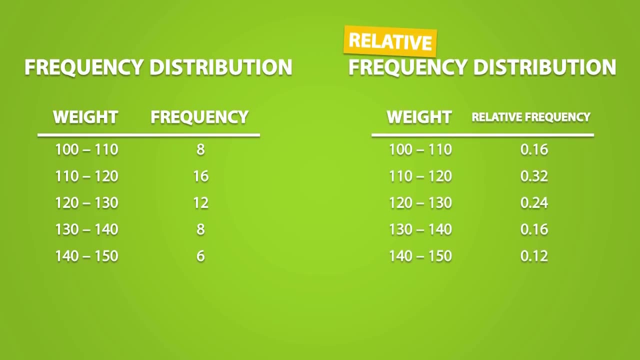 Now the problem with this is that we don't have continuity. For example, if you weighed 119.7 pounds, there would be no interval that contains this value. Now a frequency distribution can be converted into something called a relative frequency distribution. The only difference between these two is that a regular frequency distribution shows a count. 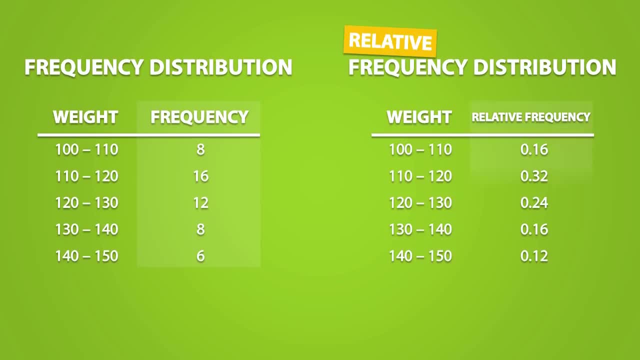 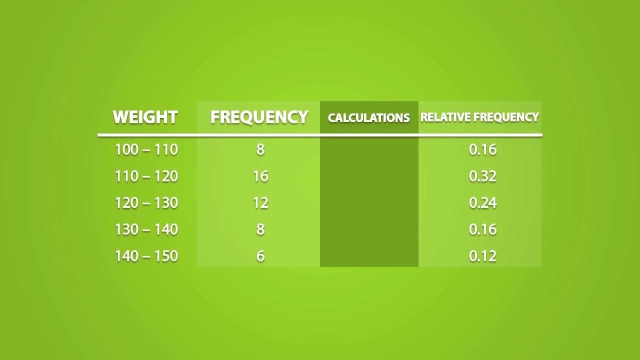 and a relative frequency distribution, as the name suggests, shows the relative frequency instead. It is called relative frequency because it represents the proportion of values in each interval in relation to the whole. To convert a frequency distribution into a relative frequency distribution we will need: 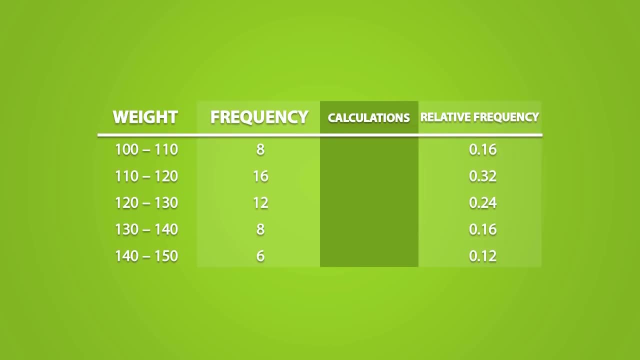 to do some calculations. We start off by finding the total number of data values, and we do this by adding each frequency. We find that the total sum is equal to 50. Then we will take each data value and add it to the total sum. 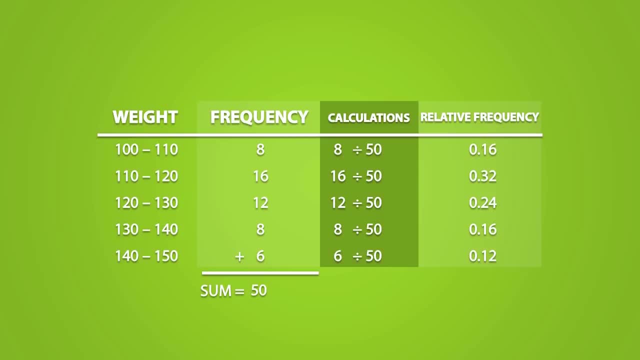 Then we will divide it by that sum And, as a result, we get the relative frequency values. To check if you have made the right conversions, you can add up all the proportions for each interval, and the sum should be equal to 1.. 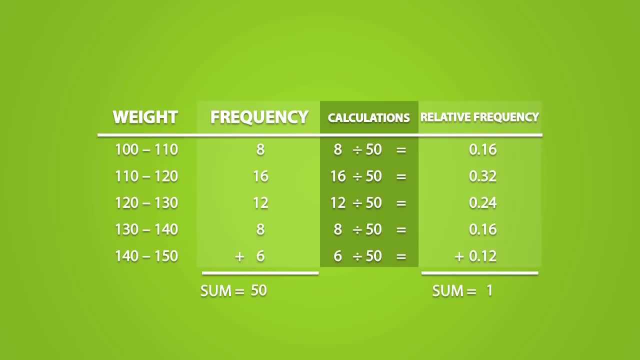 The answer should be equal to 1, because we have used a ratio that relates our data to the total amount of data values. Because of this ratio, relative frequencies can be written in percentages. To convert to percentage form, all we do is multiply each value by 100%. 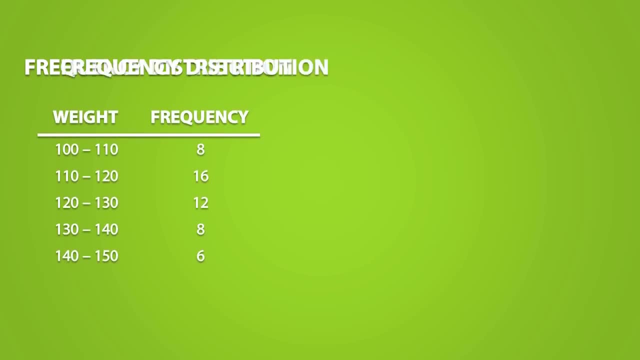 value. Now a frequency distribution can be converted into something called a relative frequency distribution. The only difference between these two is that a regular frequency distribution shows a count and a relative frequency distribution, as the name suggests, shows the relative frequency instead. It is called relative frequency because it represents the proportion of values in each. 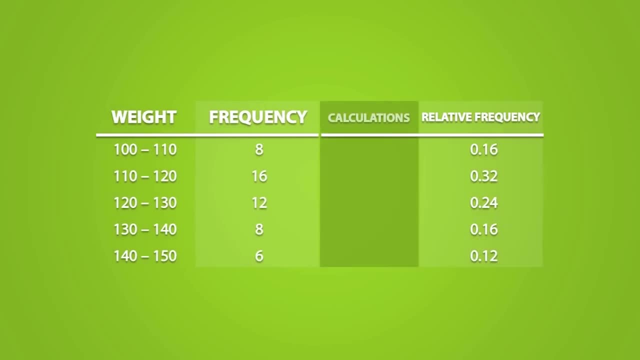 interval in relation to the whole. To convert a frequency distribution into a relative frequency distribution, we will need to do some calculations. We start off by finding the total number of data values and we do this by adding each frequency. We find that the total sum is equal to 50.. 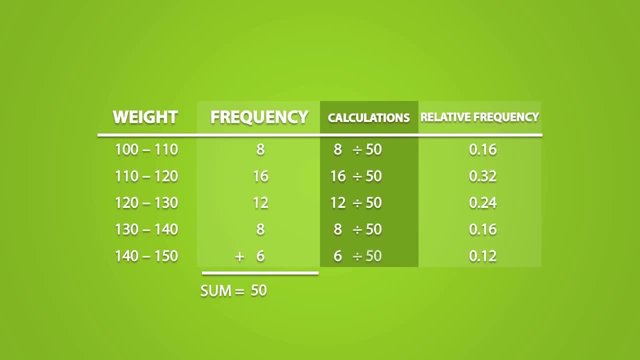 Then We will take each value and we will divide it by that sum And, as a result, we get the relative frequency values. To check if you have made the right conversions, you can add up all the proportions for each interval, and the sum should be equal to 1.. 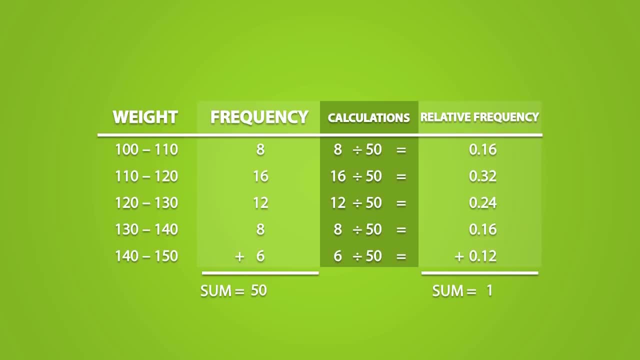 The answer should be equal to 1, because we have used a ratio that relates our data to the total amount of data values. Because of this ratio, relative frequencies can be written in percentages. To convert to percentage form, all we do is multiply each value by 1.5.. 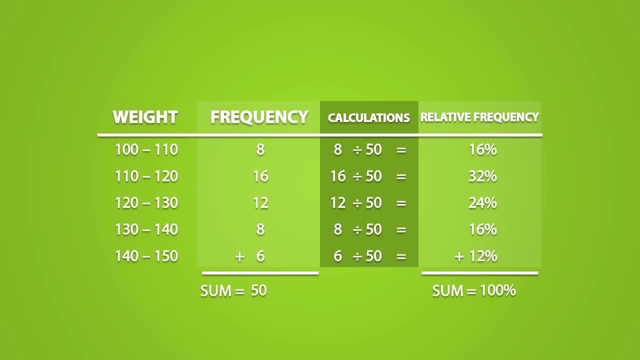 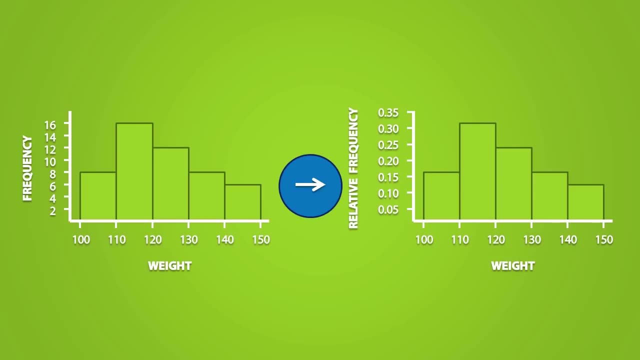 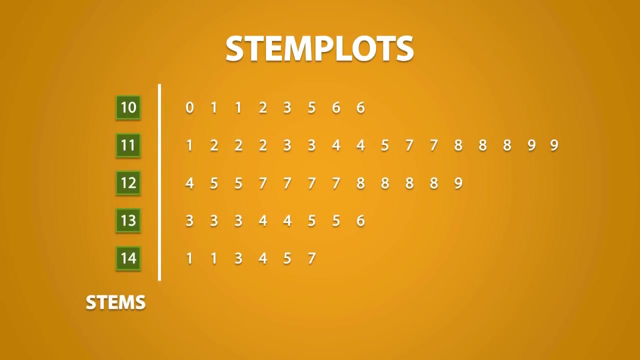 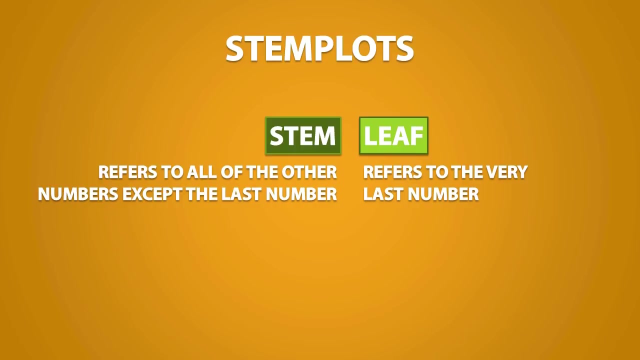 That's it. In the same way, regular histograms can be converted into histograms that tell us the proportion of values for each interval. Now, stem plots are like histograms, except they show each data point. Stem plots consist of stems and leaves. A leaf refers to the very last number and a stem refers to all of the other numbers. 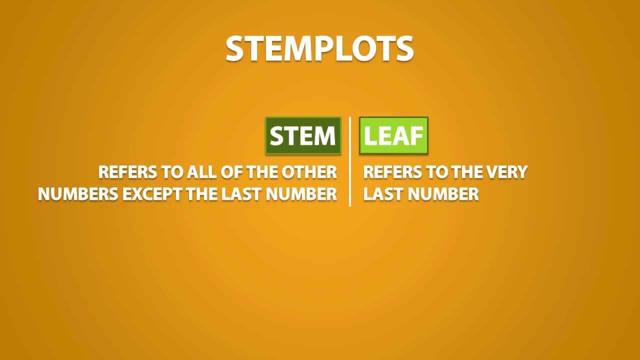 except the last number. Stems and leaves are usually separated by a line. For example, Let's look at the number 117.. The leaf is the last number, so this would be 7.. The stem is all of the other numbers, so the stem is 11.. 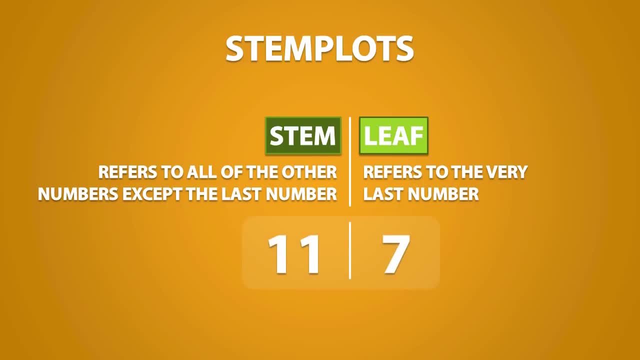 On a stem plot, this would be written as so. Now let's look at the number 69.. Using the same rules, we would get a leaf of 9, and a stem of 6. And on a stem plot, this would be written as so: 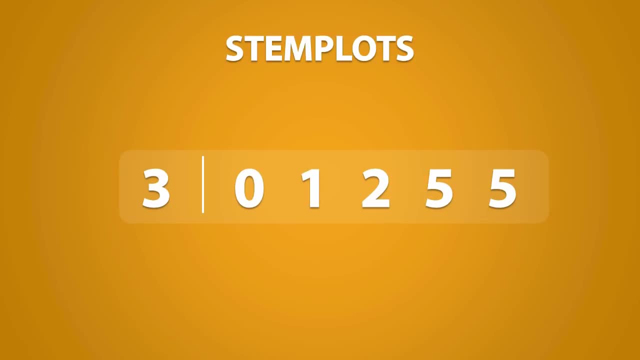 Now, when we have a string of leaves like this, it just means that I have the data points 30,, 31,, 32,, 33,, 34,, 35,, 36,, 37,, 38,, 38,, 39,, 40,, 41,, 42,, 42,, 42,, 42,, 42,, 43,, 42,, 42, 43,, 42, 42,. 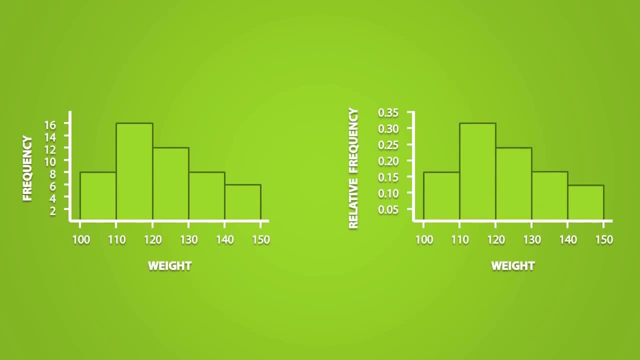 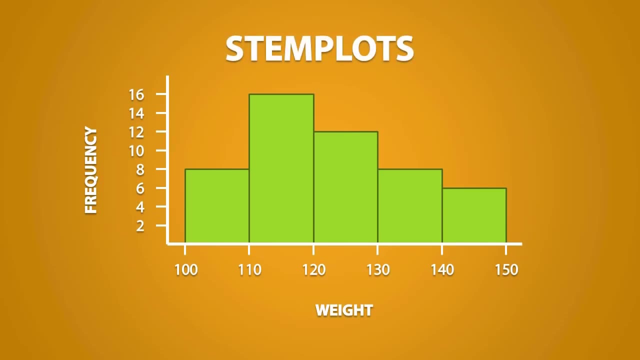 So we have the total amount of data values. In the same way, regular histograms can be converted into histograms that tell us the proportion of values for each interval. Now, stem plots are like histograms, except they show each data point. Stem plots consist of stems and leaves. 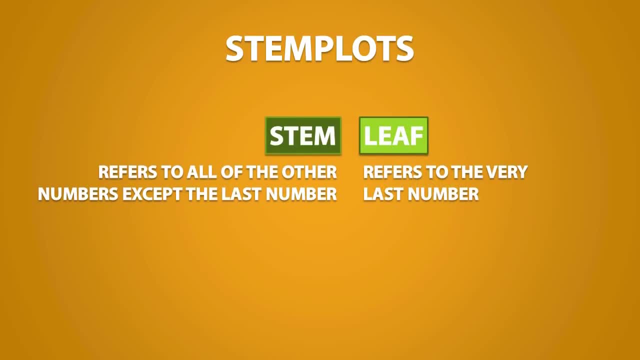 A leaf refers to the very last number and a stem refers to all of the other numbers except the last number. Stems and leaves are usually separated by a line. For example, let's look at the number 16.. The number 16 is the number of the tree. 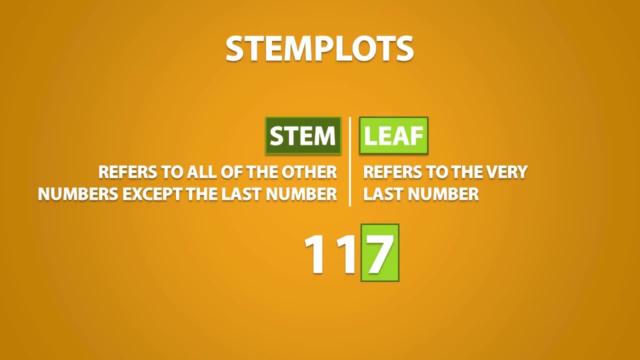 The number 16 is the number of the tree. The leaf is the last number, so this would be 7.. The stem is all of the other numbers, so the stem is 11.. On a stem plot this would be written as so: 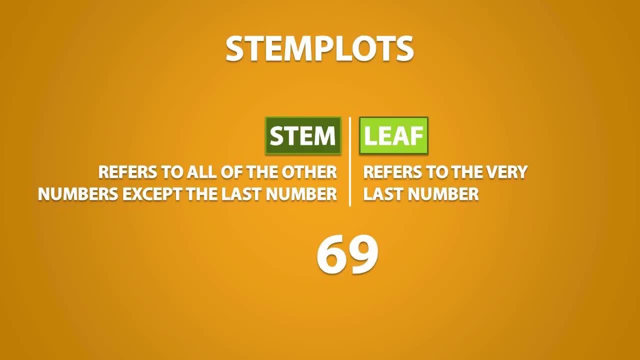 Now let's look at the number 69.. Using the same rules, we would get a leaf of 9 and a stem of 6. And on a stem plot this would be written as: so: Now, when we have a string of leaves like this, it just means that I have the data points. 30, 31,, 32, and 32.. 35 and 35. Notice how stem plots are constructed. Stems go down from low to high and leaves extend outward from low to high, Depending on the dataset we are working with. sometimes we can get stem plots with too many. 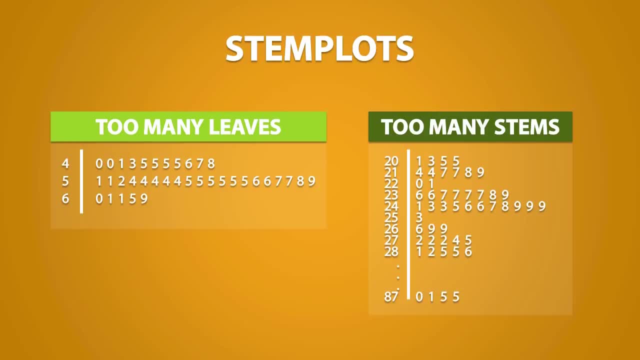 leaves and we can get stem plots with too many stems. When this happens, we might not get a nice picture of the distribution and, as a result, we may not be able to get much information out of it. This is not quite true. 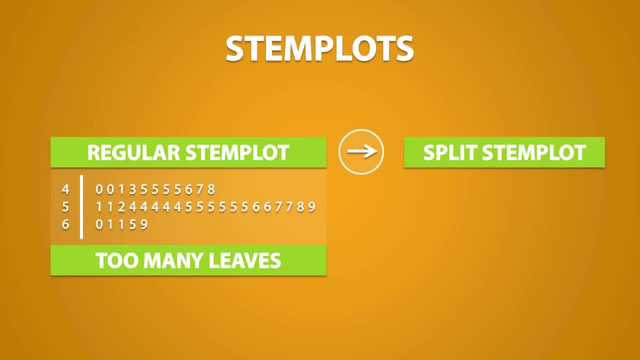 Let's say we get two leaves plot with too many leaves, we can convert it into something called a split stem plot. This conversion is called splitting the stems. To split the stems, we need to duplicate each stem. The first stem will run from 0 to 4, which corresponds to these values. 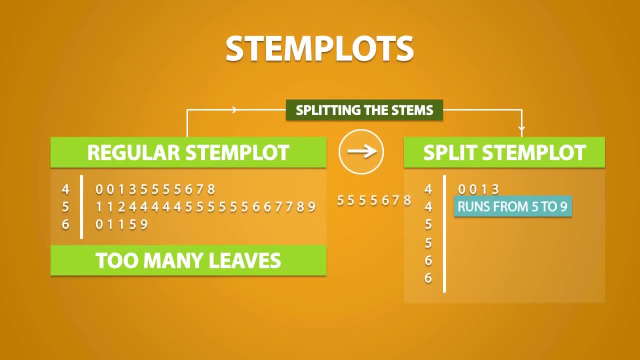 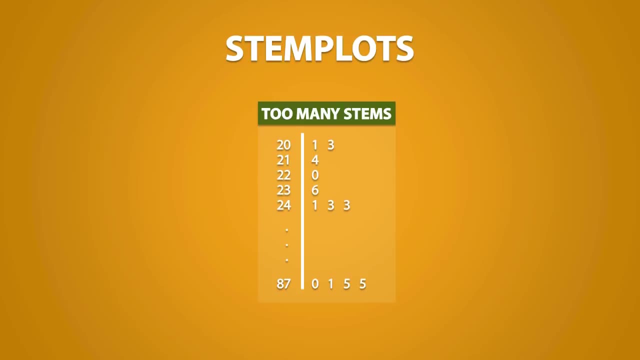 And the second stem will run from 5 to 9,, which corresponds to these values. The same logic can be applied to the rest of the stems. When we have too many stems, we can reduce the amount of stems by trimming the leaves. 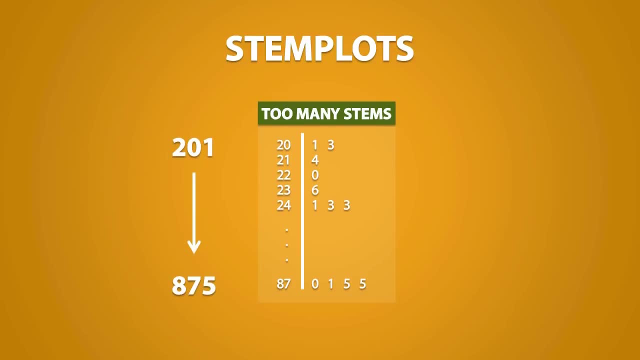 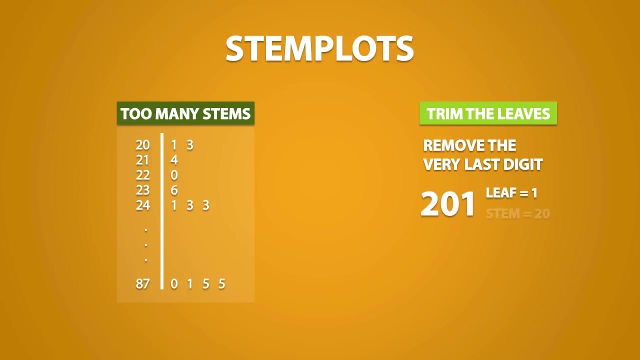 In this example we have a very large dataset that goes from 201 all the way to 875. That's over 60 stems that we have to write To trim the leaves. all we do is remove the very last digit. So notice for the number 201, the leaf is 1 and the stem is 20.. 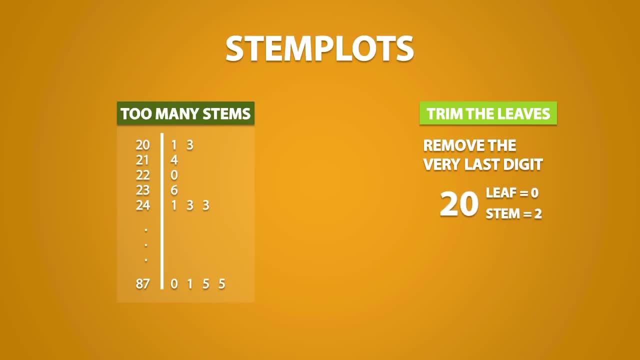 After removing the very last digit, we get 20.. So now the leaf becomes 0. And the stem is now 2.. We would do the same process for each data value. By trimming the leaves we get a better looking stem plot. 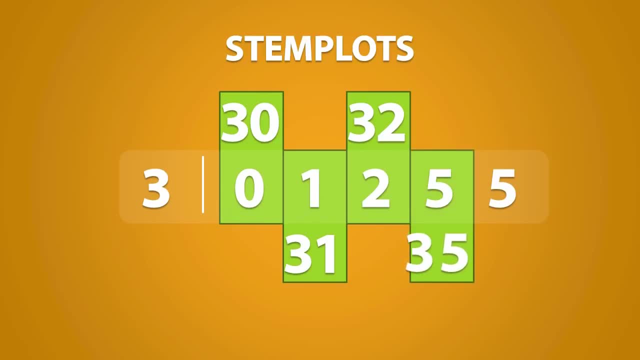 43,, 44,, 45,, 46,, 47,, 48,, 49,, 50,, 51,, 52,, 42,, 43,, 44,, 45,, 46,, 47,, 48,, 49,, 50,, 51,, 52,, 43,. 44,, 45,, 46,, 47,, 48,, 50,, 51,, 52,, 42,, 43,, 42,, 44,, 44,, 45,, 46,, 47,, 48,, 51,, 52,, 43,, 44,, 45,. 44,, 46,, 47,, 48,, 51,, 52,, 43,, 44,, 45,, 46,, 47,, 48,, 51,, 52,, 44,, 45,, 46,, 49,, 51,, 52,, 45,. 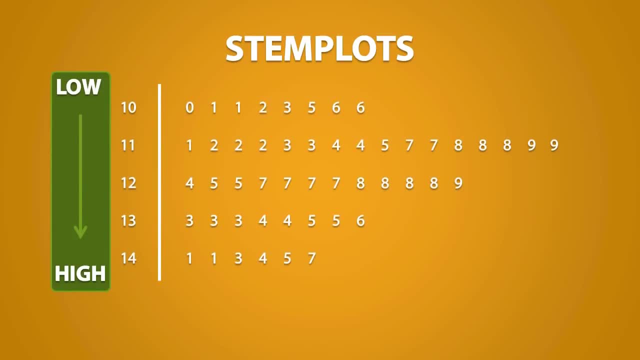 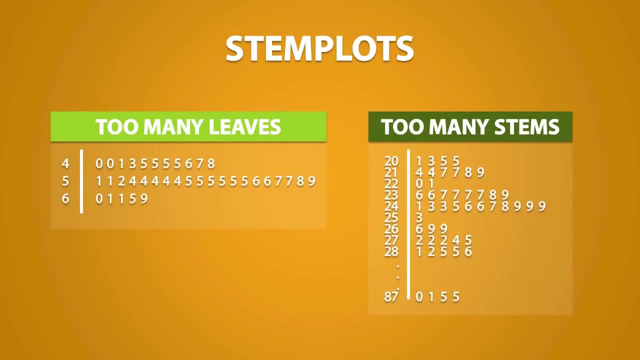 Notice how stem plots are constructed. Stems go down from low to high and leaves extend outward from low to high, Depending on the dataset we are working with. sometimes we can get stem plots with too many leaves and we can get stem plots with too many stems. 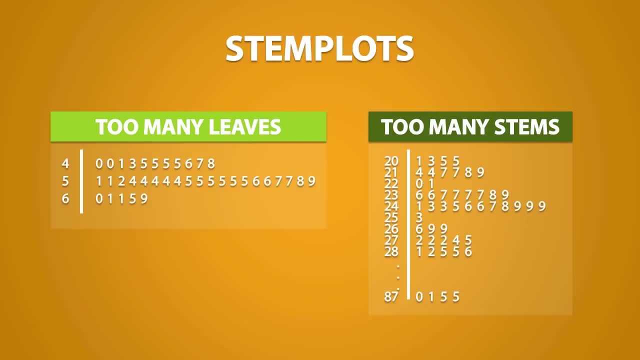 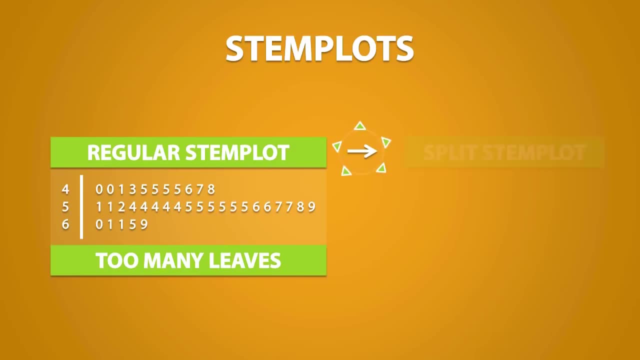 When this happens, we might not get a nice picture of the distribution and, as a result, we may not be able to get much information out of it. If we have a regular stem plot with too many leaves, we can convert it into something called. 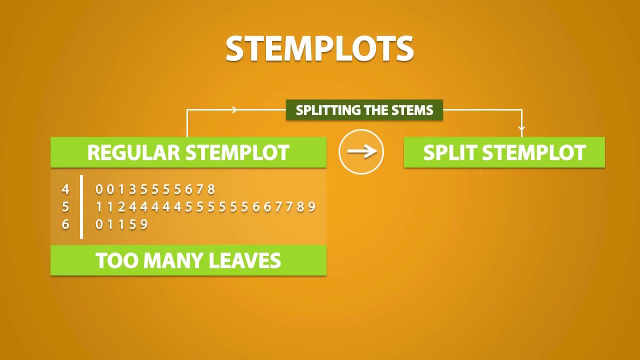 a split stem plot. This conversion is called splitting the stems. To split the stems, we need to duplicate each stem. The first stem will run from 0 to 4,, which corresponds to these values, And the second stem will run from 5 to 9,, which corresponds to these values. 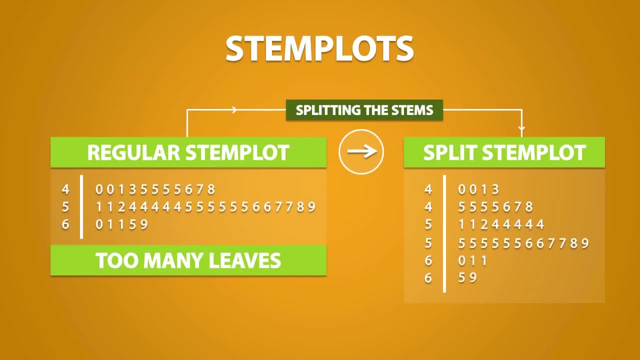 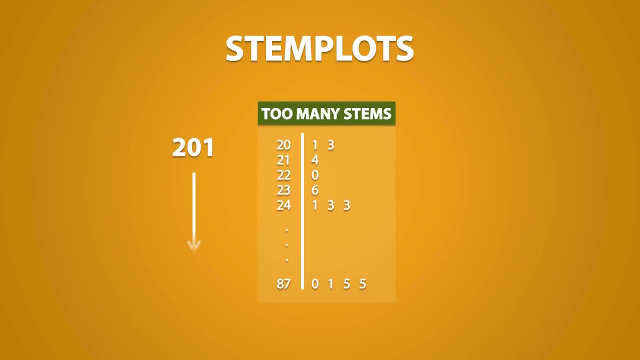 The same logic can be applied to the rest of the stems. When we have too many stems, we can reduce the amount of stems by trimming the leaves. In this example, we have a very large dataset that goes from 201 all the way to 875.. 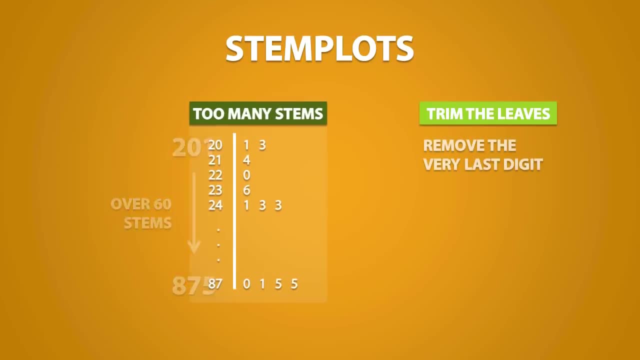 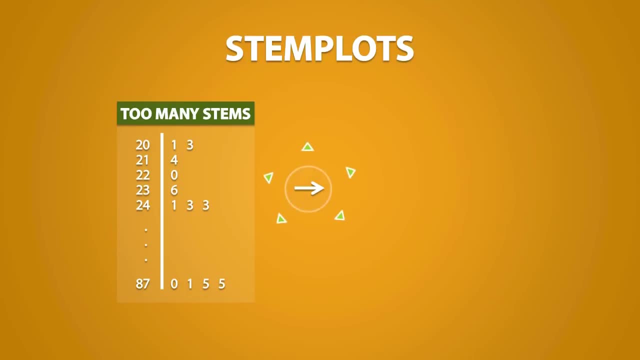 And the stem is now 2.. We would do the same process for each data value. By trimming the leaves, we get a better looking stem plot. Notice how we have reduced the amount of stems by doing this And we have saved ourselves the trouble of having to write down over 60 stems. 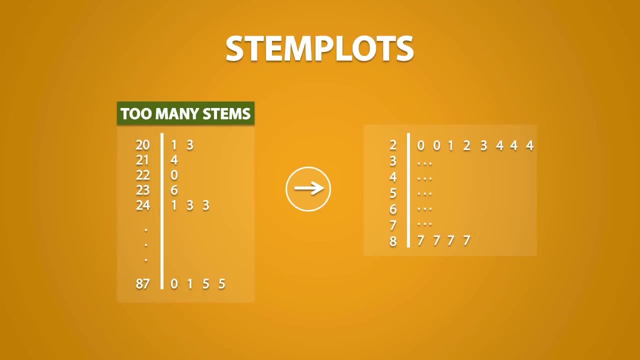 Notice how we have reduced the amount of stems by doing this And we have saved ourselves the trouble of having to write down over 60 stems. This is why trimming can be useful, But be careful when you read this stem plot after it has been trimmed. 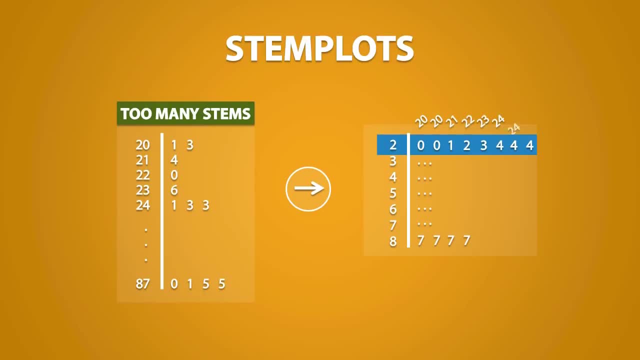 For example, for the top row. instead of reading it as 20,, 20,, 21,, 22,, 23, and so on, We want to keep the stem somewhat lower. we read it as 200,, 200,, 210,, 220,, 230, and so on. 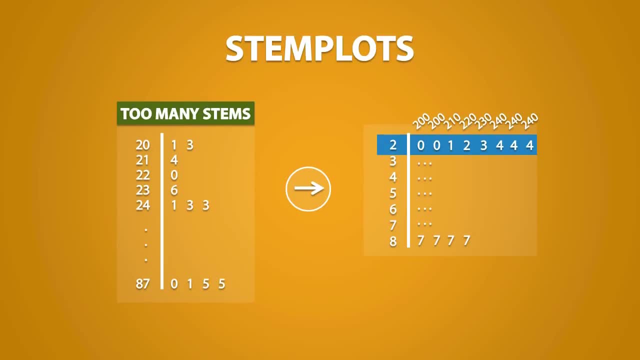 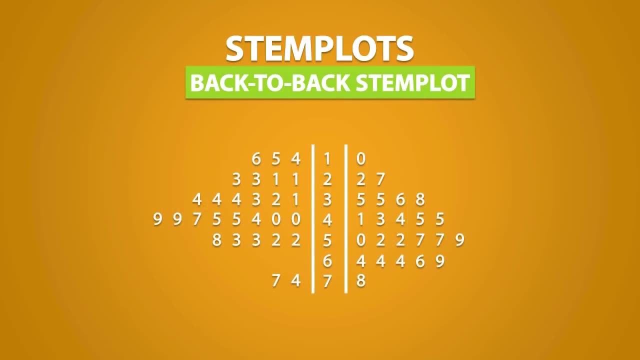 This is because the original data was in the hundreds place. Now the last type of stem plot we will be looking at is called a back to back stem plot. Back to back stem plots are used to display and compare two distributions by using the same set of stems. 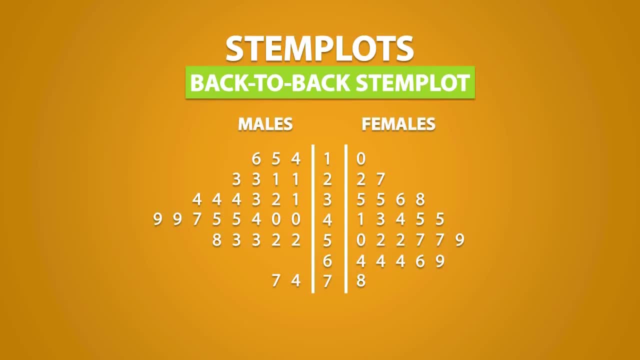 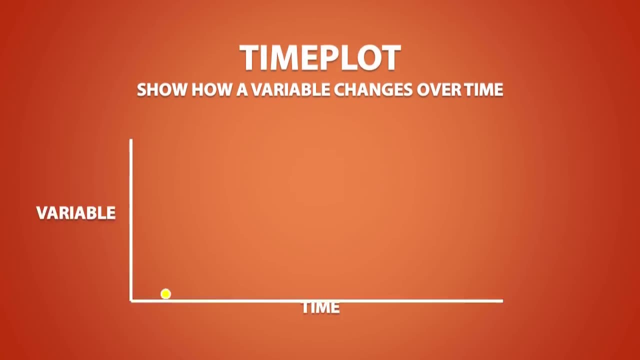 So, for example, we could compare data from males and females, or data from cats and dogs. Another way to display quantitative data is by using a time plot. Time plots show how a variable changes over time. By convention, time is always plotted on the x axis and the values of a variable are always 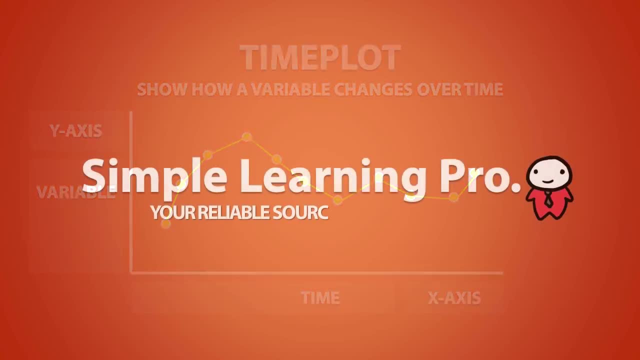 plotted on the y axis. 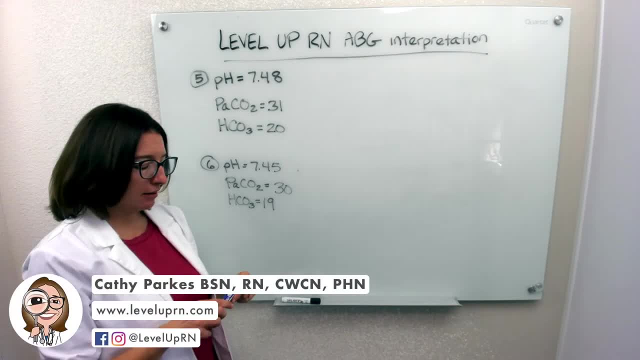 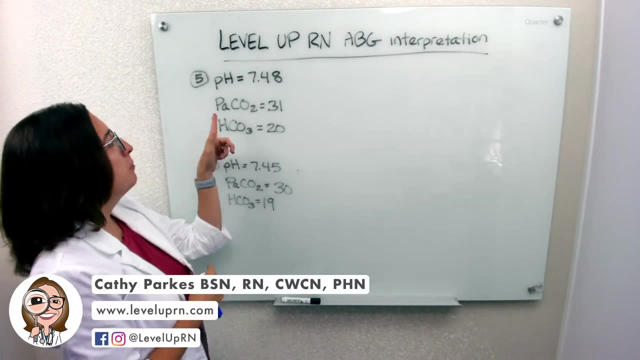 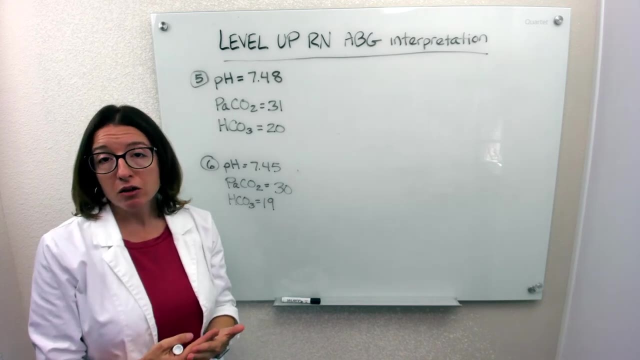 All right, we're going to work through some more ABG problems. I have a new pen so hopefully that'll work better. Number five: we have a pH of 7.48,, PaCO2 of 31,, HCO3 of 20.. First step: do we have acidosis or alkalosis based on the pH? pH should be between: 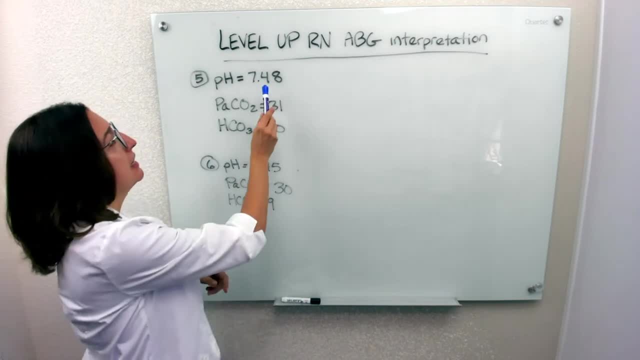 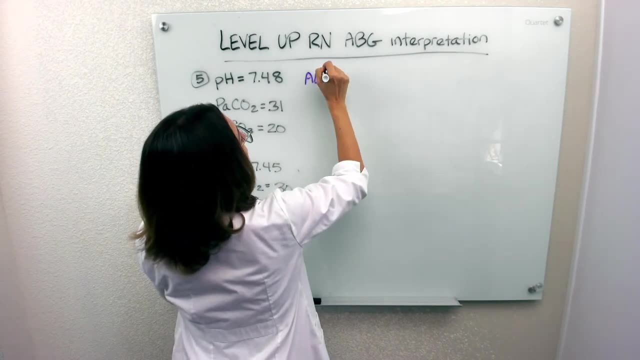 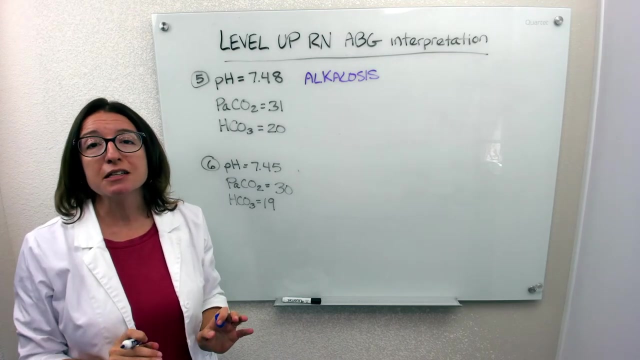 7.35 and 7.45.. Because it is out of range. on the high side we know we have alkalosis. So that is step one. Step two: who's the blank? The respiratory system or the metabolic system? So let's look at PaCO2 to. see if it's the respiratory system acting up. So PaCO2 should be between 35 and 45.. 31 is out of range and it's out of range on the basic side. So we know right away that we have respiratory alkalosis. So I'm going to write that down here. 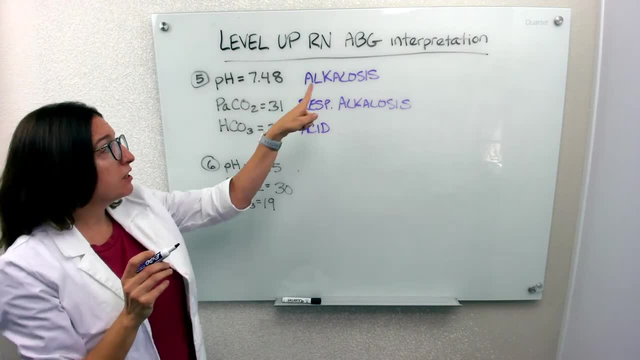 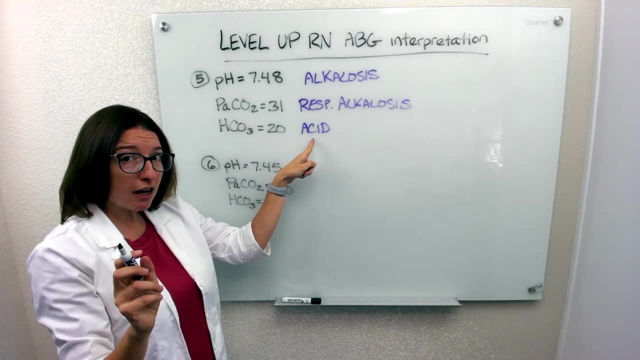 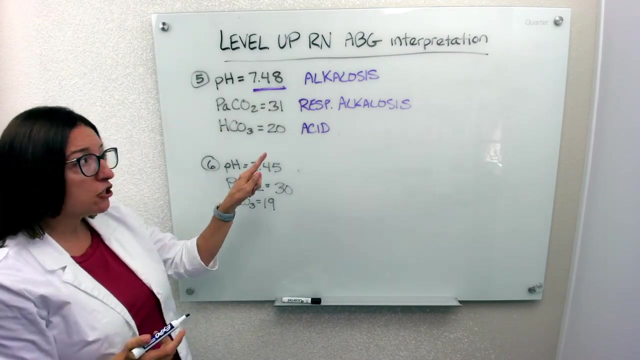 Let's see how that goes. So we have respiratory alkalosis. We have the metabolic system trying to compensate, but it is not fully compensated because our pH is out of that normal range. So in this case we have partially compensated respiratory alkalosis. So write that up here.